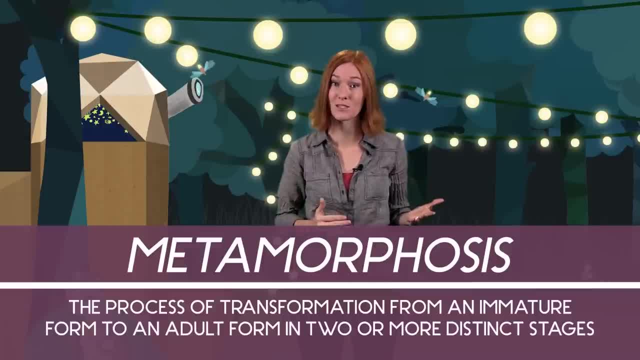 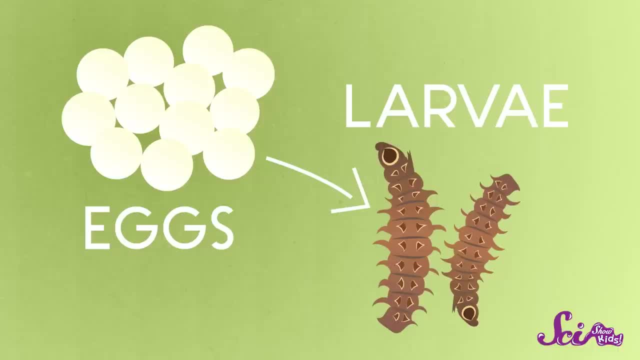 Metamorphosis is the series of changes that take place over a certain animal's life cycle. Fireflies begin as eggs. Female fireflies lay their eggs underground, where they hatch and become larvae, And both an egg and a larva of a firefly can glow just like an adult. After about a year, the larvae move into the next stage of metamorphosis, called the pupa stage. This is where the insects gradually change from looking like long, lumpy larvae into the adults that we recognize After they reach adulthood. fireflies only live for a few months. 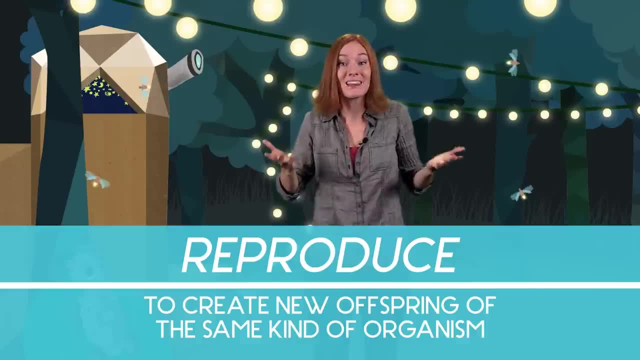 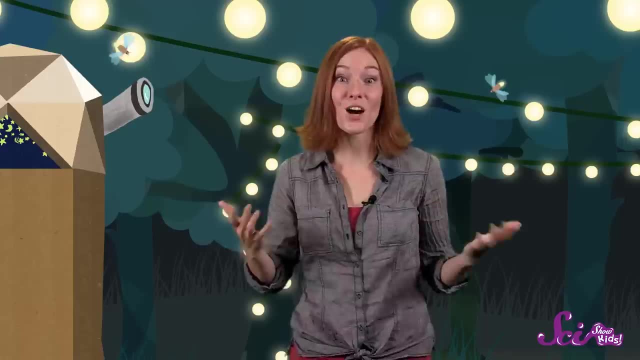 This is just long enough for them to reproduce lay eggs and start the life cycle all over again. And what fireflies eat depends on what part of the life cycle they're in: Larvae, since they live underground, eat things like snails and slugs, while adult fireflies eat pollen and nectar from flowers. 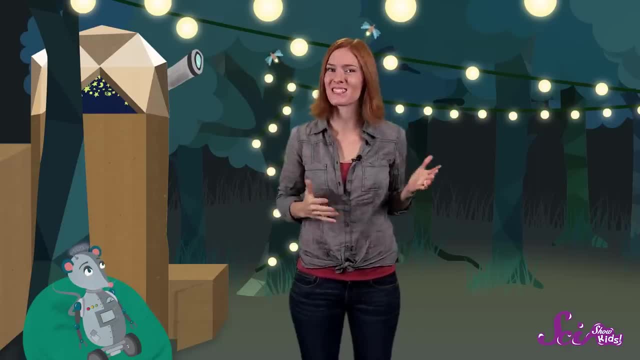 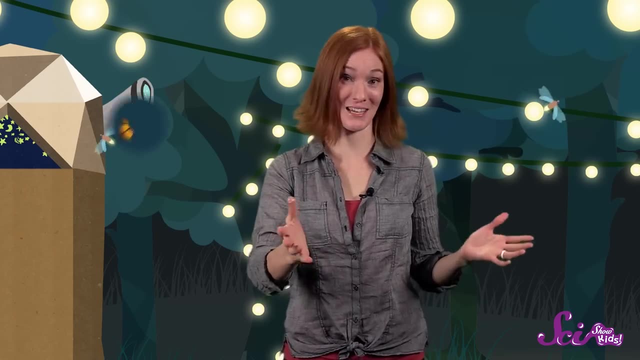 Or sometimes other fireflies. Still other adult fireflies seem to eat nothing at all. Some scientists think this might be because they live for such a short time, And since fireflies and other beetles are insects, you know what that means. 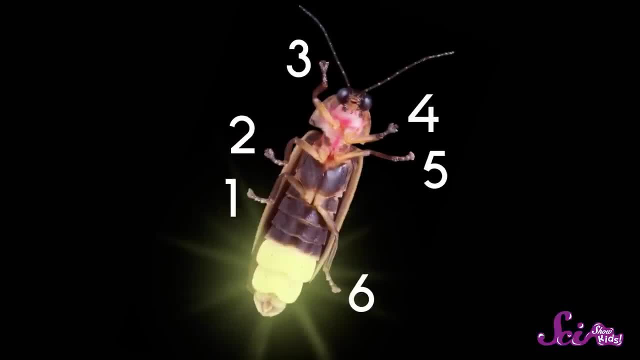 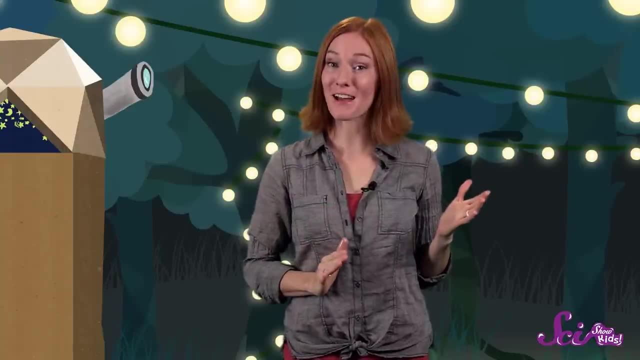 It means fireflies have what all insects have in common: They have six legs and they have three main body parts: The head, the thorax and the abdomen. And it's what goes on beneath the firefly's abdomen that makes it different from most other insects. 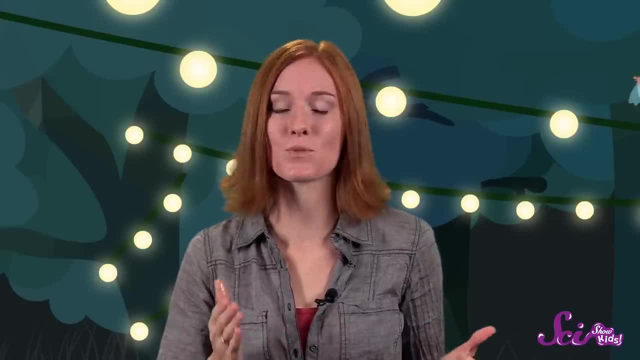 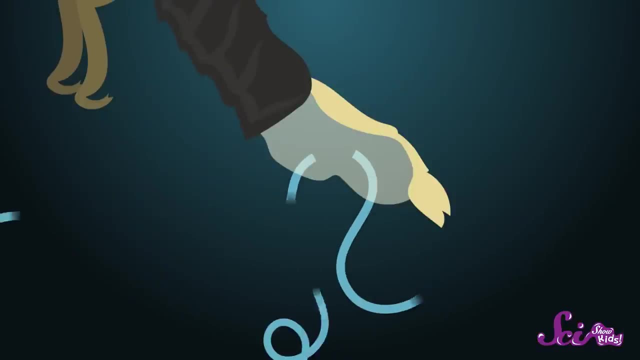 Fireflies have a special body part beneath their abdomens that does one thing: It makes light. When oxygen from the air enters this part of the body, it mixes with special chemicals inside, causing the firefly to glow. Scientists call this glow bioluminescence. 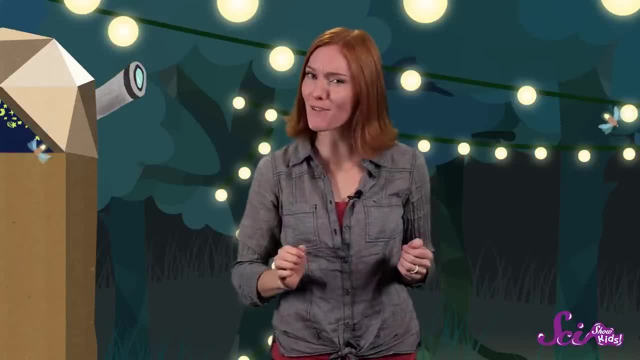 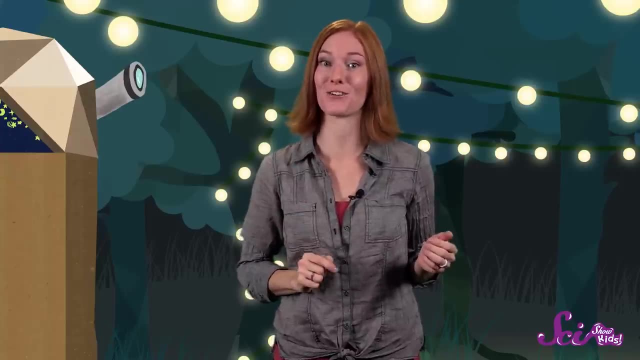 It comes from a living thing. Scientists know how bioluminescence works in fireflies, but they're not quite sure how the insects are able to turn it on and off in a specific pattern. That's a question that they're still studying. 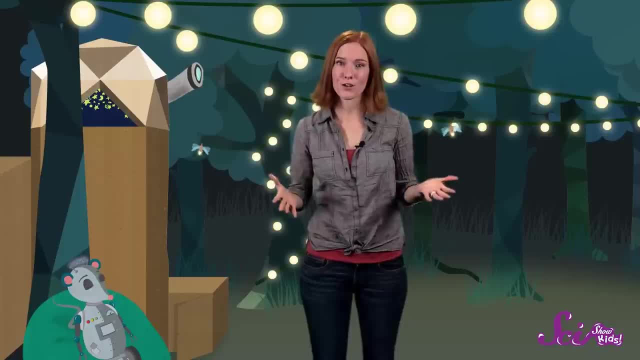 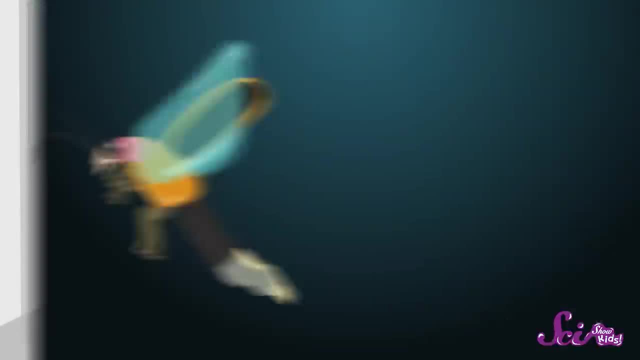 But scientists do know a lot about why fireflies flash. First. flashing probably sends a warning to predators. just like some flashing lights send warnings to people, A firefly's light sends a message to hungry animals that their glowing bodies taste bad, so they should stay away. 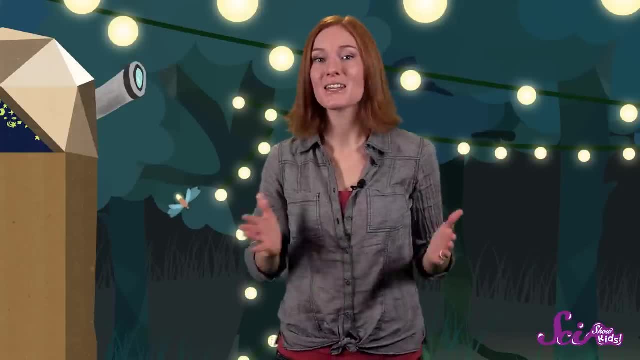 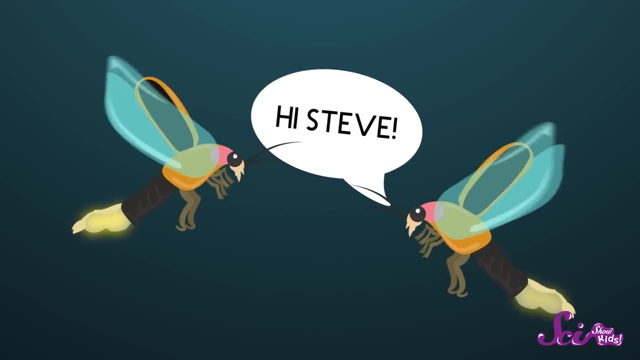 Flashing is also a way that fireflies communicate with other animals. They're able to communicate with other animals. The blinking pattern might tell other fireflies not to get too close to their homes, or it might help fireflies that are of the same kind or species to identify each other. 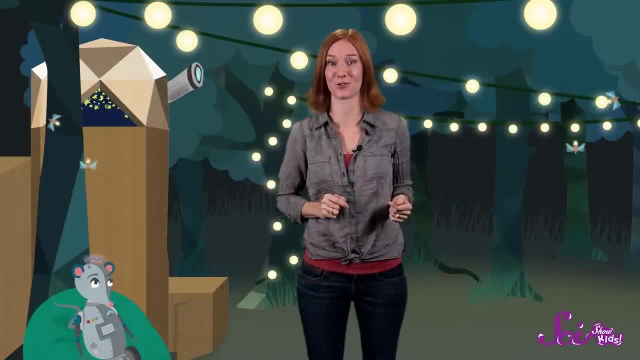 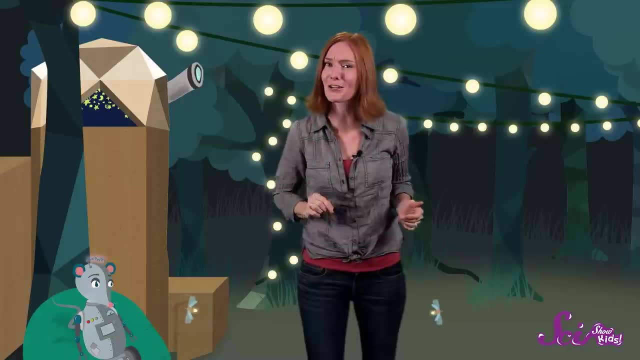 And sometimes the flashing might be a signal that one firefly sends to another to attract a mate. In many kinds of fireflies the female can't fly. Instead she'll cling to a leaf or a branch, flashing her light when she sees a male fly by.